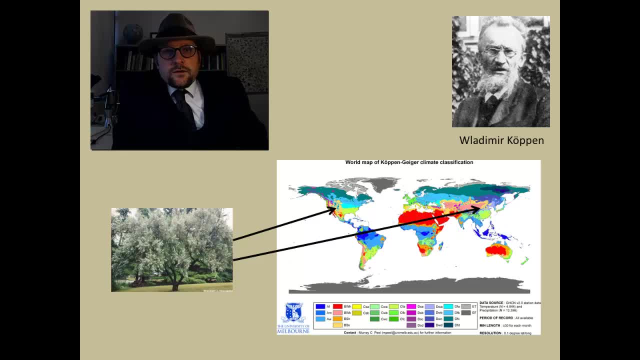 Let me explain how this would work. This is the Russian olive tree, and if you live anywhere in the American west, you have likely seen this plant, which is an invasive plant that was brought over from Asia, where it grows on the Russian Basin. It is a plant that grows on the Russian Basin, which is 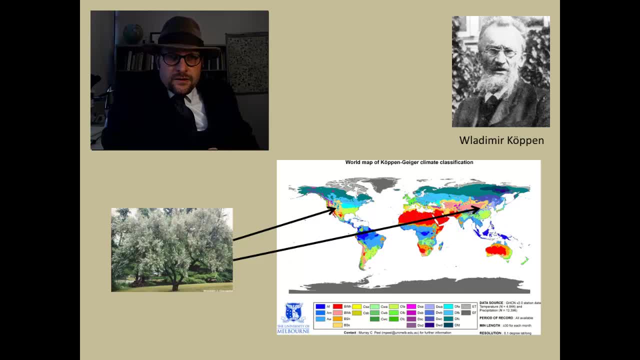 It is a well adapted plant for the harsh, hot and dry summers and freezing cold temperatures of the Russian steppes as well as in the American west. hence it is found in the same Copland classification zone. so here it is shaded in pink and you notice that there is. 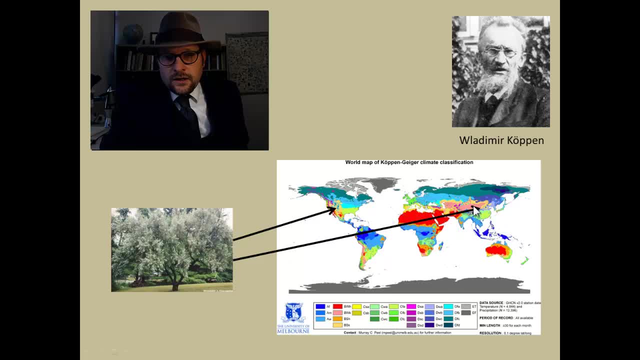 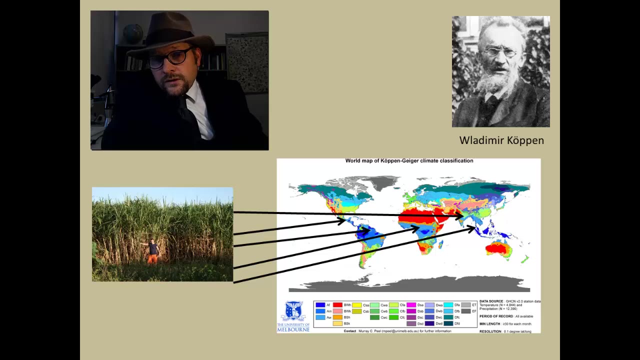 the same classification over here in North America as there is in the Russian steppes. You would expect the Russian olive tree to grow in any of these areas on the map. This is sugarcane, our most important source of sugar. Sugarcane grows in the Copland zone that is colored light blue. so Copland's classification. 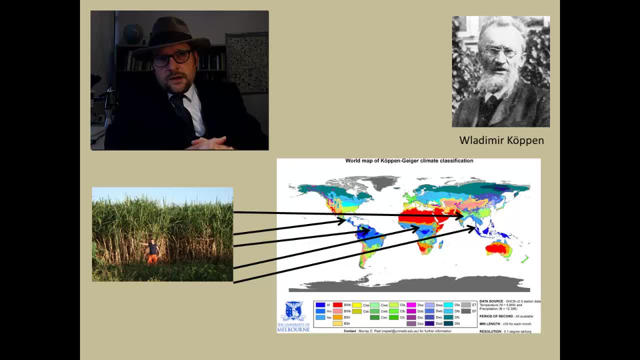 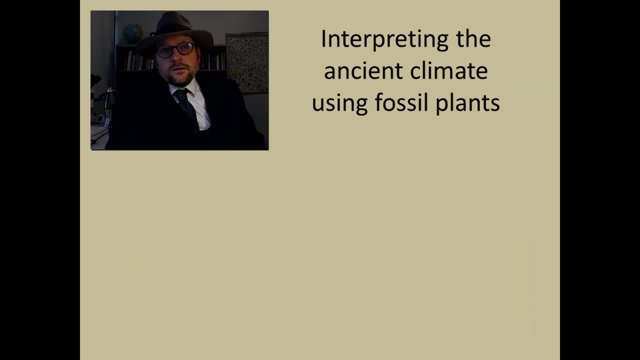 had a very real and important purpose. Plants are adapted to particular climatic conditions. The question that Copland asked was that could fossil plants be used in a similar way to infer past climates on the Earth at various geological periods of time? Copland proposed this idea over 100 years ago. 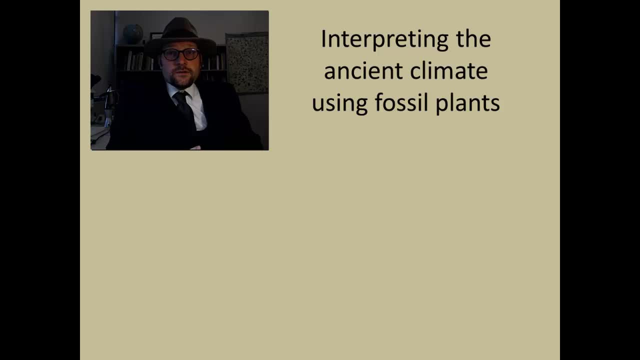 Today in this lecture, we will examine three ways to use fossil plants to interpret ancient climates in the geological past. The first technique is what Copland first proposed, using what is called the co-existence model or the nearest living relative model. In the last 50 years, more sophisticated models have been developed: the climate leaf analysis. 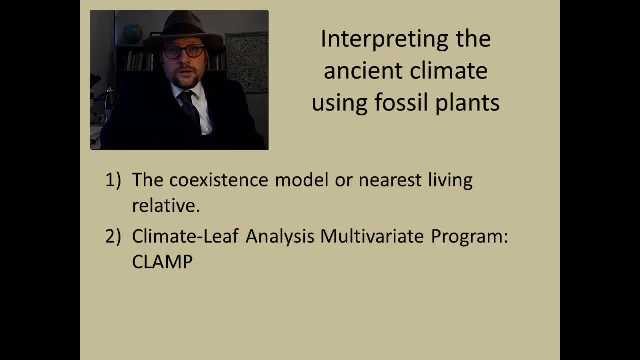 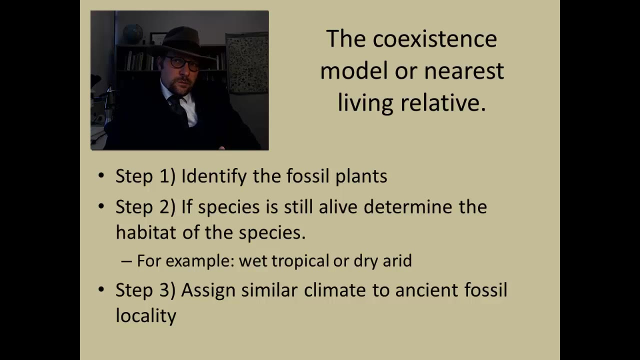 multivariate program, CLAMP and the more modern leaf margin analysis. So let's take a look at the earliest technique that was developed, the co-existence model, first. The co-existence model has three steps. The first is to identify the fossil plants that we find in the fossil record. 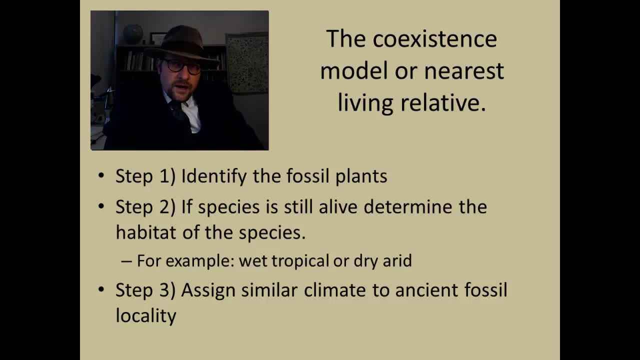 Second, if the species is living, we can look at the habitat of the living plant. For example, does it live in wet tropical environments or does it live in dry, arid environments today? Next, we can assign a similar climate to the ancient fossil locality. 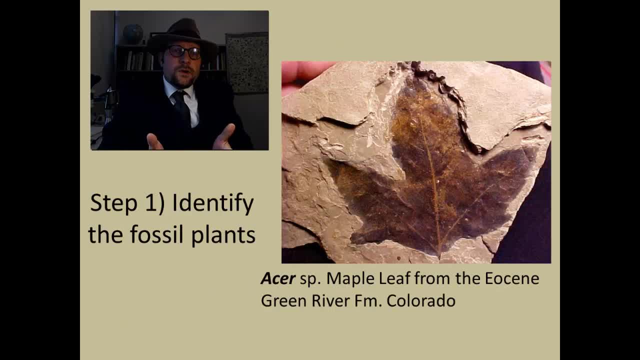 Let's take a look at an example of how this would work. So here we go. we have a fossil from the southern Rocky Mountains of Colorado out of the Middle Eocene Green River. The fossil is identified as belonging to Acer, a genus for maples, and indeed it looks very. 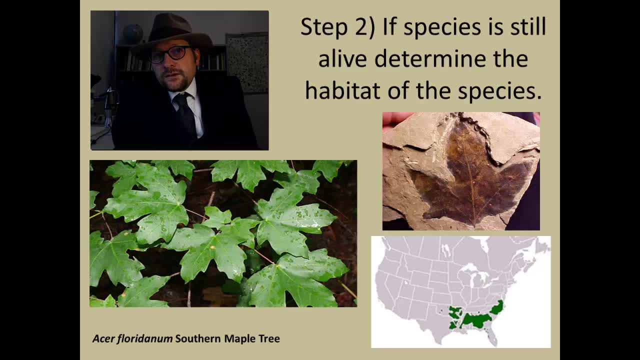 similar to modern maple leaves. The modern southern maple tree, Acer floridum, lives in the more wet and warm southeastern part of the United States today and none are known living in the Rocky Mountains today. So, looking at its modern distribution, We can assume that the climate 50 million years ago in Colorado would be similar to 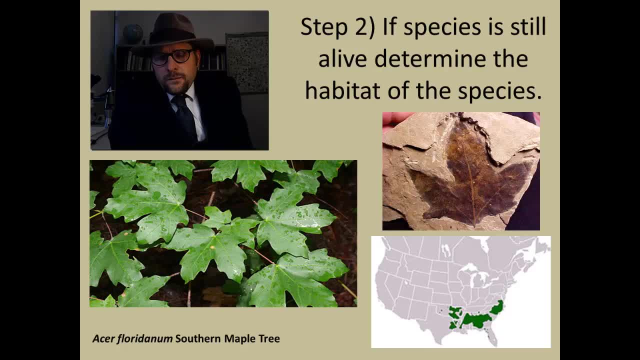 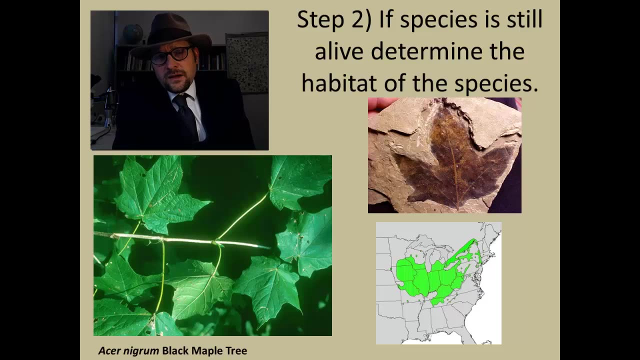 that in Georgia and Mississippi today, But we need to be very careful. here. Is our fossil really a member of this species? This is the black maple tree, Acer nigrum, and it also looks a lot like our fossil leaf and it grows in the much cooler climate, similar to Illinois and southern Michigan. 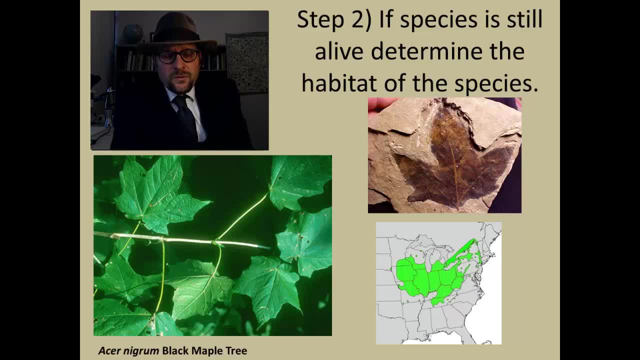 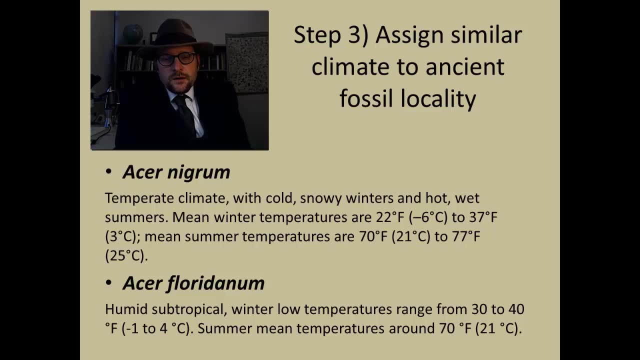 It grows in the much cooler climate, similar to Illinois and southern Michigan. So was the climate in Colorado more cold or warm? This is one of the big problems with using the coexistence model. Depending on how confident our identifications are, it can have a really powerful effect. 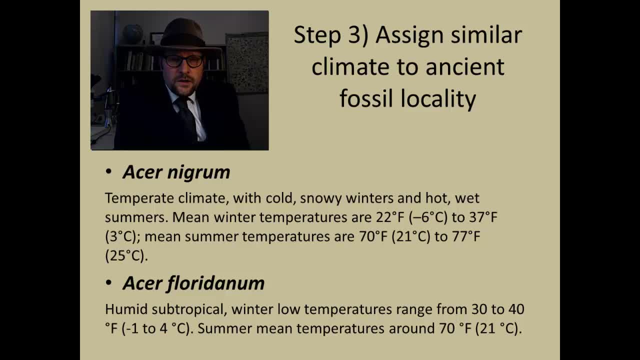 on the resulting climate range we reconstruct from the past. If our fossil belongs to Acer nigrum, we would interpret a temperate climate with cold, snowy winters and hot, wet summers. Mean annual winter temperatures are around 22°F or negative 6°C, so below freezing. 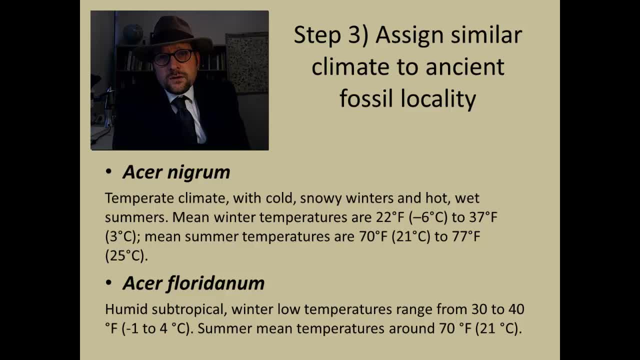 to 37°F or 3°C, with mean summer temperatures in the 70s to high 70s and high 20s. If the fossil belongs to Acer floridum, We would interpret a humid subtropical climate never getting much below freezing so low. 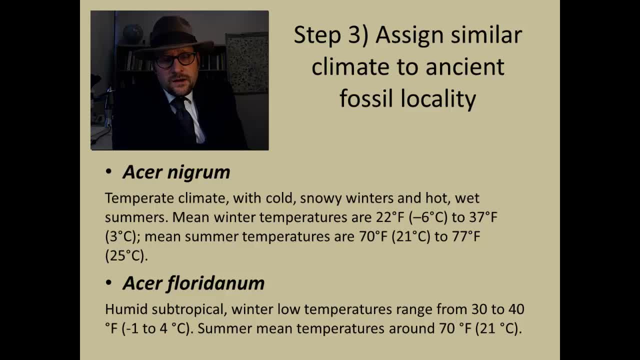 temperatures in the winter ranging from about 30°F to 40°F, with mean summer temperatures around 70°F to 20°C. So that is a pretty big difference between these two, Just depending on how we identify the fossil. Another problem comes up if there is no living species for the fossil. 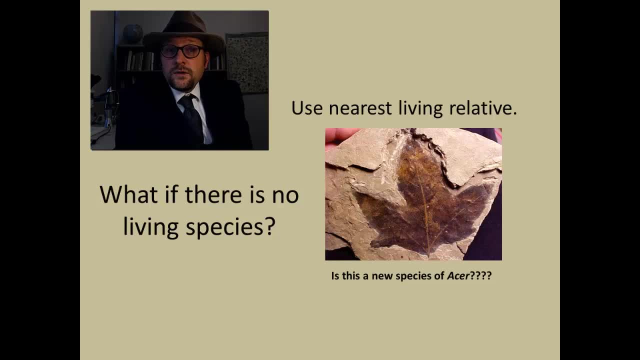 Maybe the fossil is a new species that is not living today. so we would have to try to interpret what that might be. Another problem comes up: if there is no living species of the fossil, Maybe the species is a new and different species than the living maples. then it would be for. 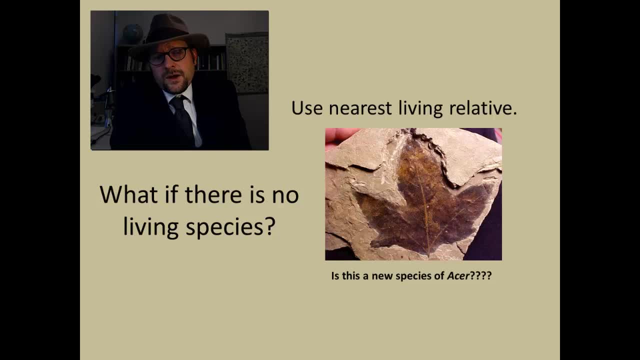 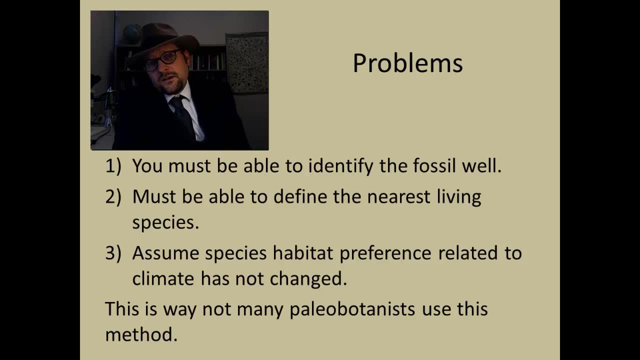 a loss. We could only speculate at what the climate might have been like. Here are some of the problems: First, you must be able to identify the fossil. second, you must be able to define what that nearest living species might be. and third, you must assume that the species' habitat. 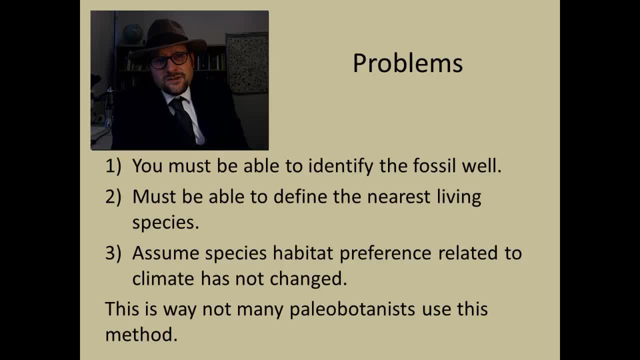 preferences related to climate has not changed over that long period of time Since its proposal over 100 years ago. not many paleontologists use this model anymore. Modern paleontologists have been using this model for a long time. They have been using this model for a long time. 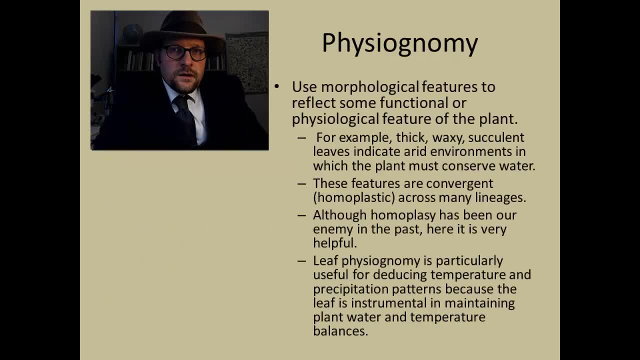 Many paleontologists, rather, have been looking at something called physiogramy. Physiogramy uses morphological features that reflect some functional or physiological feature of the plant. For example, many plants that live in desert environments will have thick waxy succulent. 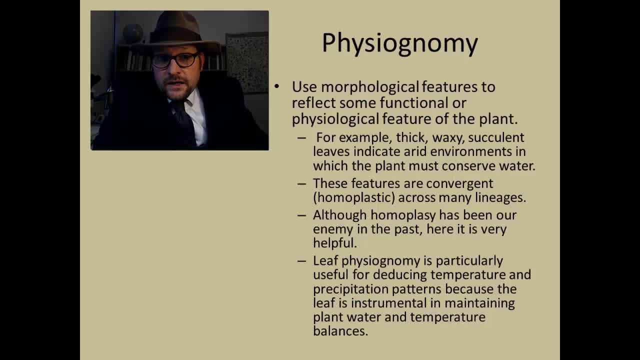 leaves to help the plant conserve water. Finding a fossil plant with these features would indicate a dry desert environment. These features are convergent, homoplastic, across many lineages. Although homoplasty has been our enemy in the past, here it is very helpful. 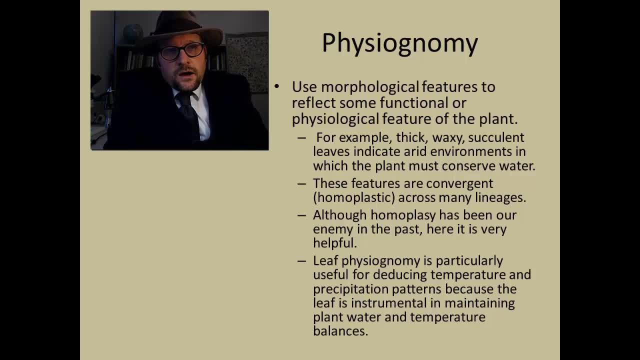 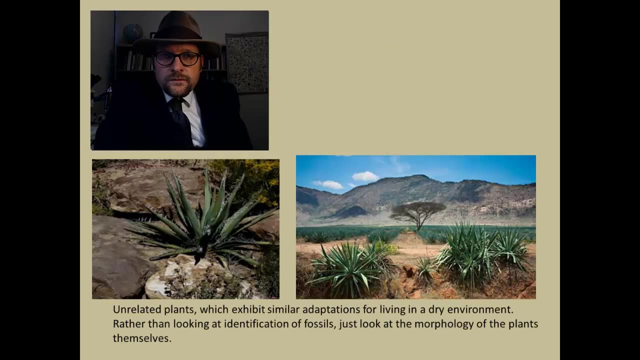 Plants don't have to be related to each other, so leaf physiogramy is particularly useful for deducing temperature and precipitation patterns, because the leaf is instrumental in maintaining the plant's water and temperature balances. Today we can see this in practice when we visit similar climates on Earth. 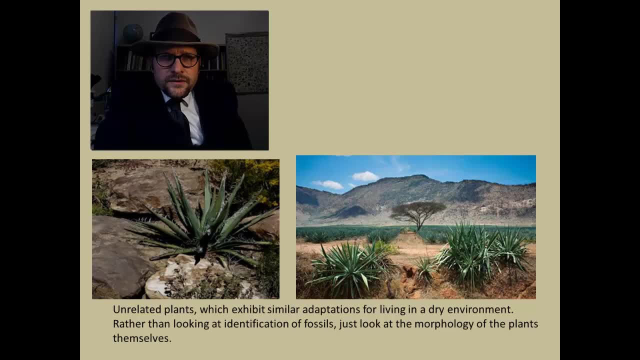 But this is not the case here. Plants live in different climates on different continents. Often the plants will superficially look similar because they are adapted to that particular climate, Such as these unrelated plants which exhibit similar adaptations for living in a dry environment. 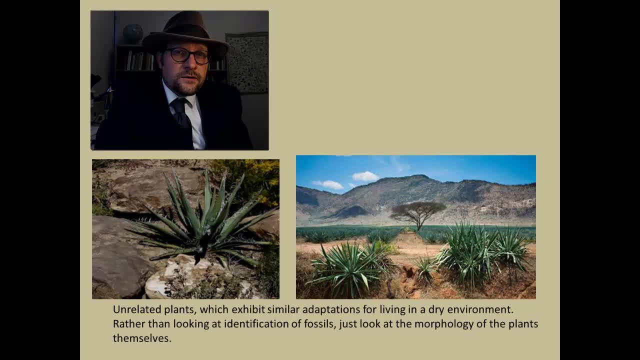 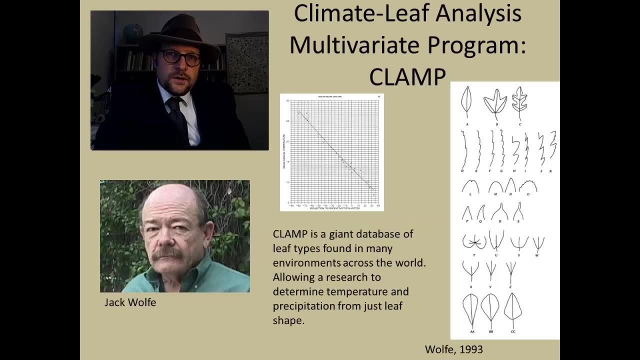 Rather than looking at the identification of the fossils, we can just look at the morphology of the plants themselves. One of the first paleontologists to use this in figuring out past climates using fossil leaves was the American paleontologist Jack Wood. He traveled the world collecting modern leaves and entering them into a database of their 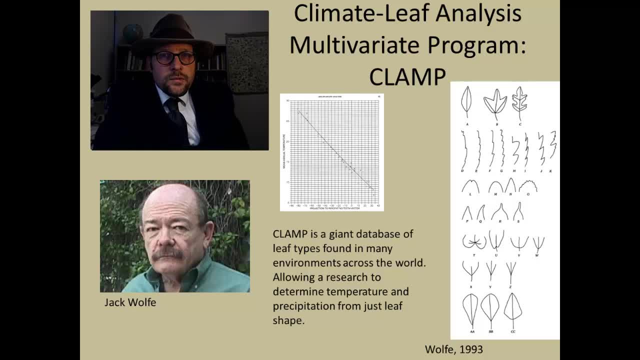 forms and shapes. He constructed a complex way of codifying these shapes into a multivariate database with many categories for leaves. In 1993 he published a monograph explaining how to conduct what he called CLAMP, which stood for Climate Leaf Analysis Multivariate Program. 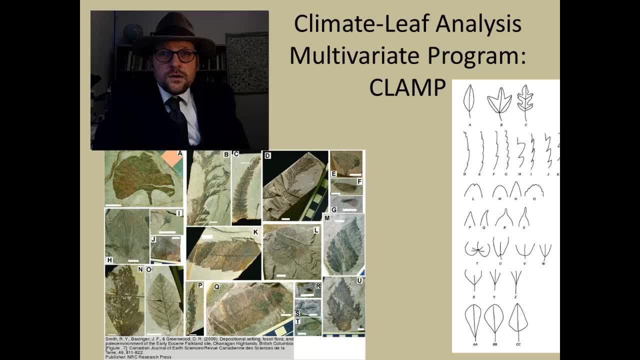 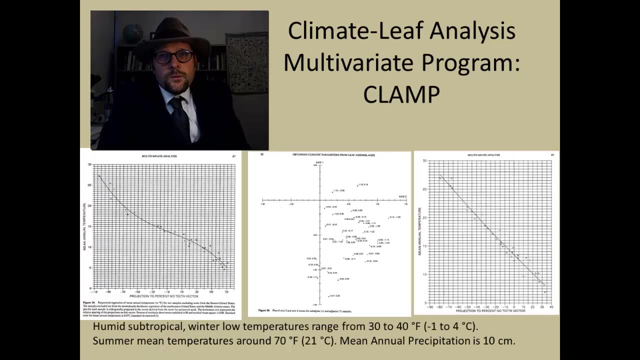 Here is how it would work: A paleontologist would assemble a collection of fossil leaves from a locality. These leaves, each one, would be codified into a database based on the occurrence of various key shapes and sizes of the leaves. Using this large database of modern leaf shapes, the program would spit out an estimate of 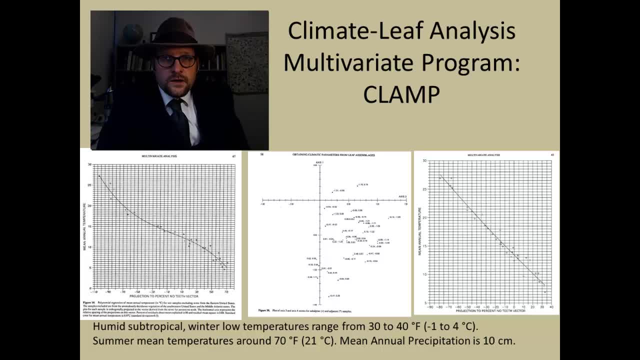 the ancient environment based on these shapes and appearances. For example, it would spit out humid, subtropical winter, low temperatures ranging from 30 to 40 degrees F. In the summer, temperatures would be around 70 degrees Fahrenheit, 21 degrees Celsius. 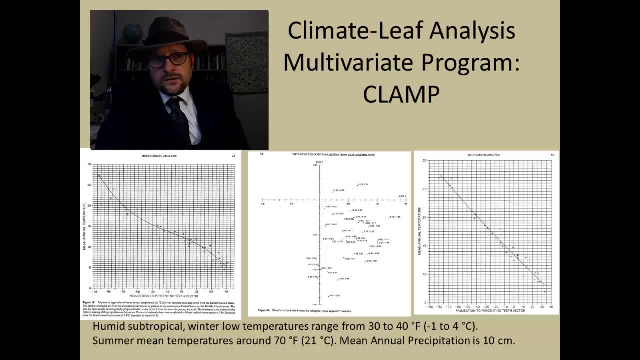 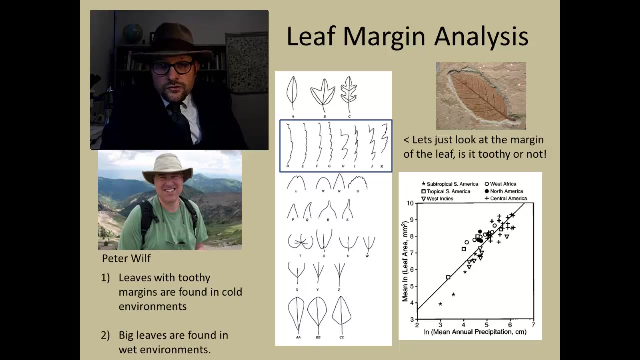 Mean annual precipitation at 10 cm a year. What is so amazing about this was that we got mean annual temperatures and precipitation estimates for the geological past. It was pretty amazing, but it required a lot of work in coding all of those leaves. Later, paleontologists realized that the complex database contained a few traits that really 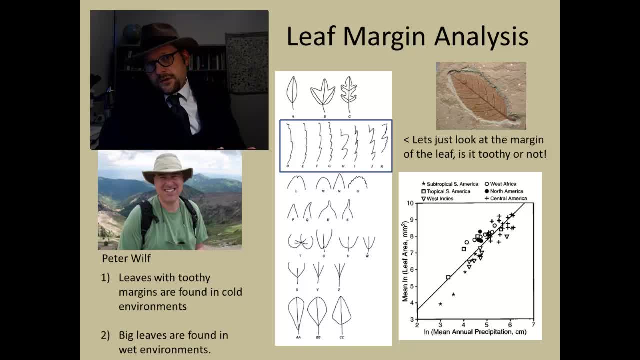 had the most effect on temperature and precipitation. Peter Welff noticed that simply looking at how toothy the leaves were gave a good estimate of temperature. More toothy margins are found in colder climates, As well as overall size of the leaves.